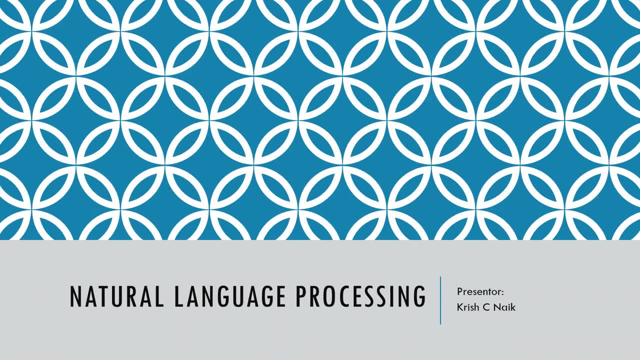 review is a positive sentiment or a negative sentiment. But how can a machine learning model can understand whether that review is a positive sentiment or a negative sentiment? Because it is not a human. It cannot understand sarcasm. So for that purpose we basically use natural. 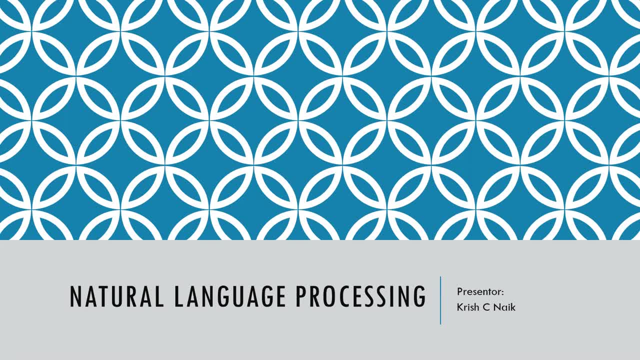 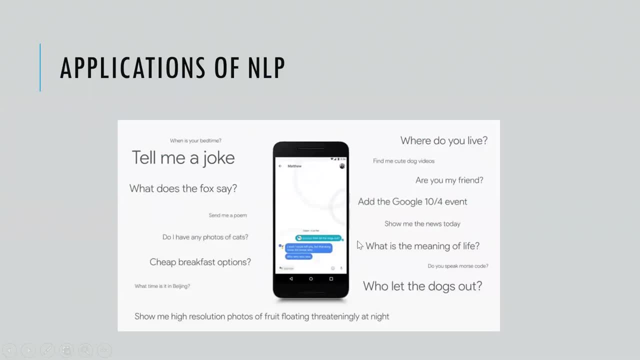 language processing. There are different kind of text processing that we usually use to handle those kind of scenarios. One of the very most recent application of natural language processing is basically the use of Google Assistant in phones, right in our smartphones. Some other examples. 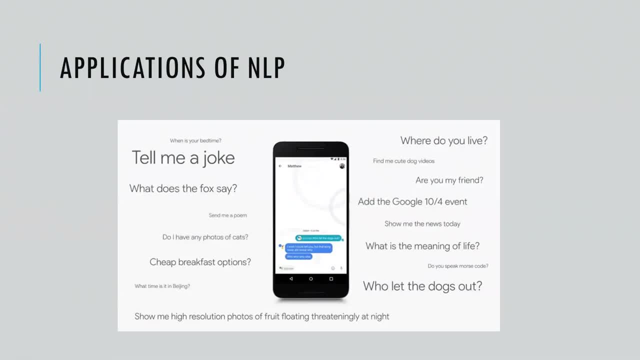 are Sri, that is used in iPhones, And you have also heard of Google Assistant. You have heard of Amazon Alexa. So these are some of the examples. With respect to applications, I hope everybody remembers Gmail. right, Many of them uses Gmail In Gmail. I think you have heard of something. 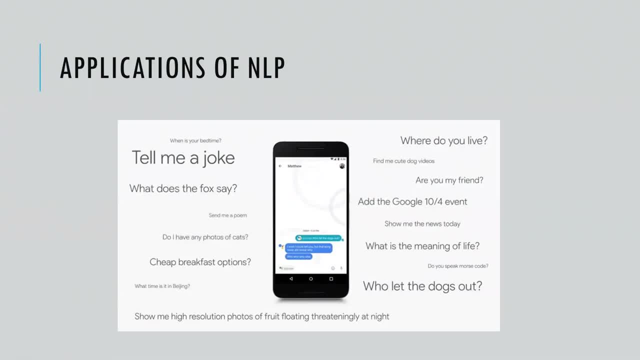 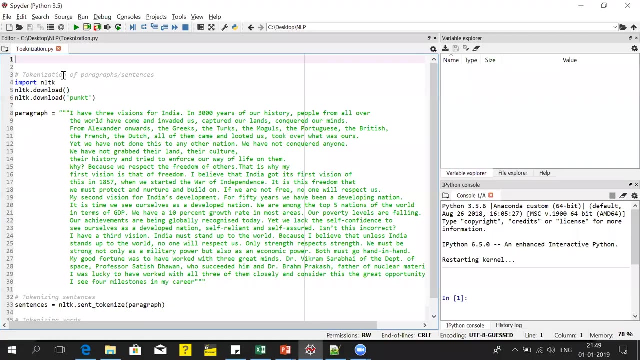 called a spam classifier. So spam classifier works completely based on natural language processing. So in this playlist we'll be completely discussing about natural language processing- all best practices that are actually used for doing text processing, and we'll be discussing all the scenarios. NLTK is a very good library that is present in natural language processing. 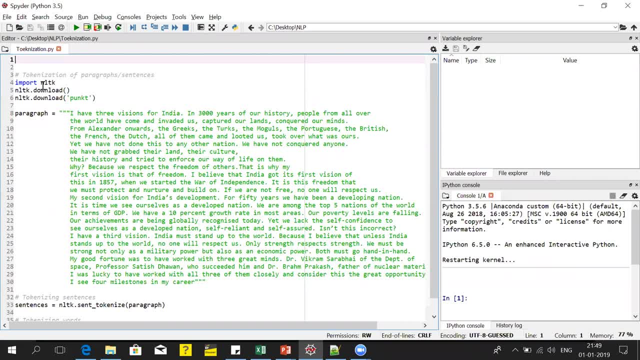 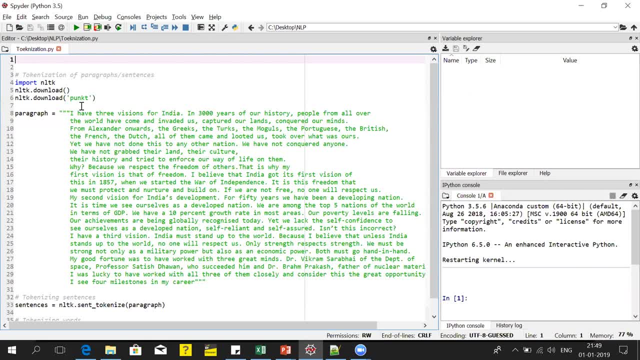 arten, Never mind. Okay, That's perfect, I got into it now. take it Now. take all of this stuff, Okay. So another theme regarding tokenization we will be talking about in a moment. Okay, So one thing that I talked about in the beginning is that when you have 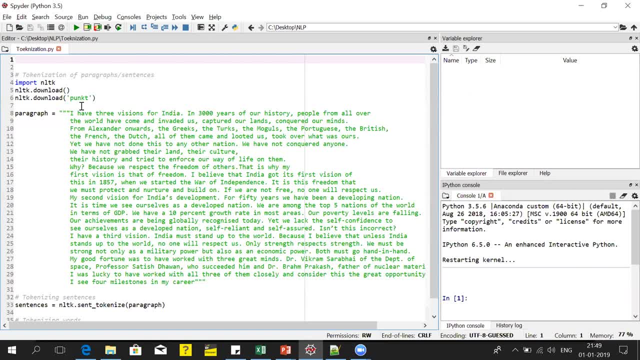 your tokenization set up. you basically have to have a separate list of what's called paperwork that you have to've set up right. So, for example, we have the daily papers As one of the key items that I've already discussed today that you need more space. there are three. 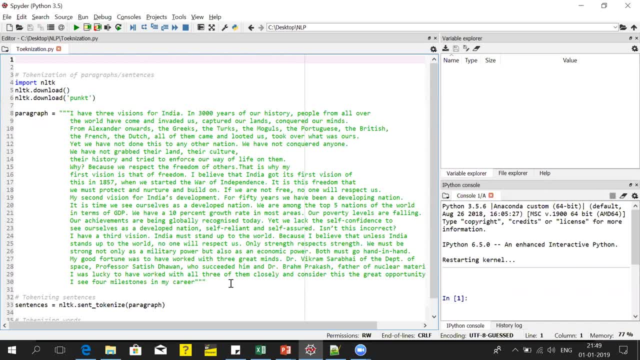 hours of miejs and all of those archaeological data filesخت, etc. and now another one. and uh, and this was the speech that was written and that was actually spoken by him, and one of the recent, you know, in one of the seminars in iit. so this was the speech that is taken and we'll try. 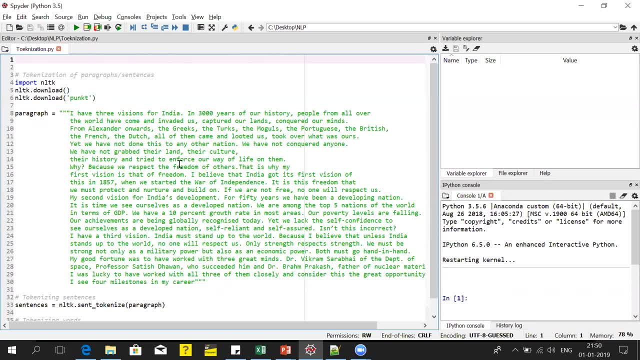 to take this particular speech and we'll try to apply different kind of text processing in this particular speech. so always the first step is basically to import the nltk. so once i import the nltk, this library is the most important library because all the text pre-processing will be using this particular nltk library. now, after importing the library, it will take some. 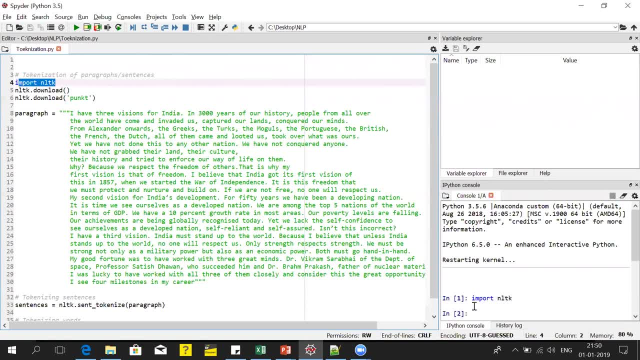 time and just let us wait till this gets executed. now you can see that this has got executed successfully. as soon as we import nltk, the next step is that we need to download all the libraries inside nltk. so once i execute this, okay, in the right hand side you'll see that there will be a 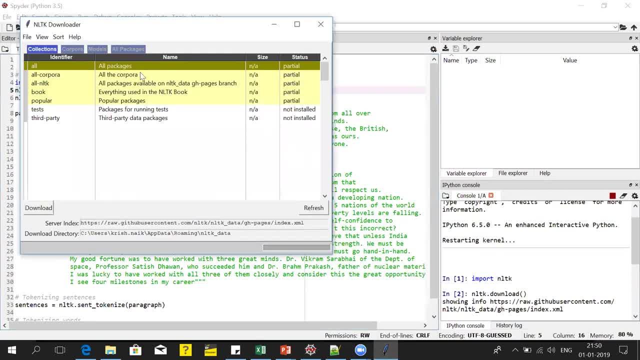 pop-up that will be nltk. so once i execute this, okay, in the right hand side you'll see that there will be a pop-up opening. okay, you click this pop-up and you can see all the packages that are present inside nltk. the first step is always: you just click the first identifier. that is all that is. we are just 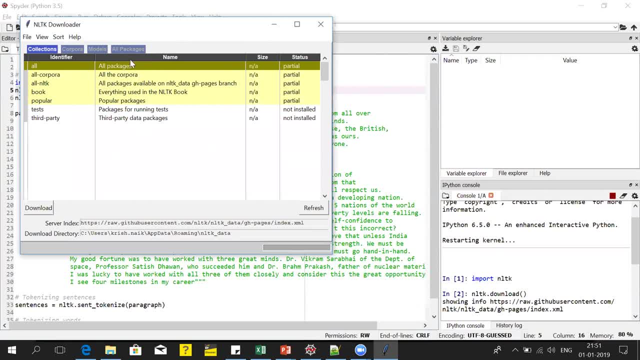 considering all the packages, so you don't have to download it again and again after clicking on this. you just click on this download button. okay, as soon as you download this, all the packages will be downloaded from this particular server index or server url and it will be downloaded inside. 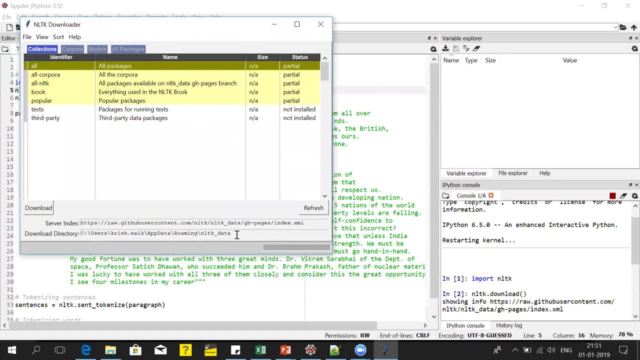 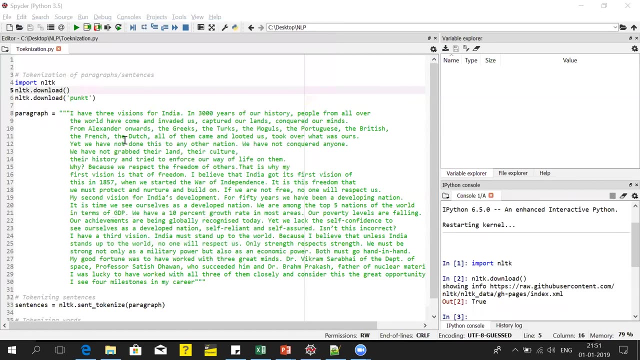 your local data well, where your anaconda is actually installed. so just to perform this particular step before you do the text pre-processing, because all the packages are present inside this nltk and you have to download it manually by using nltkdownload. i'm not going to download it because i've already. 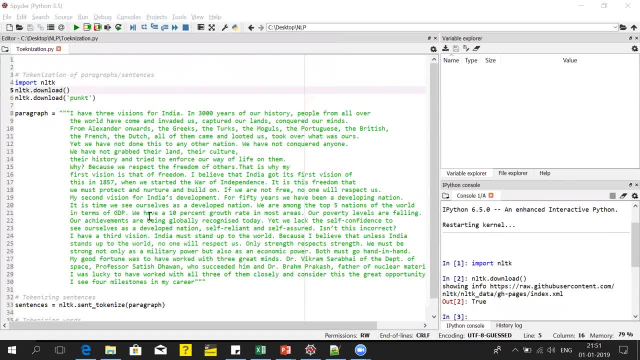 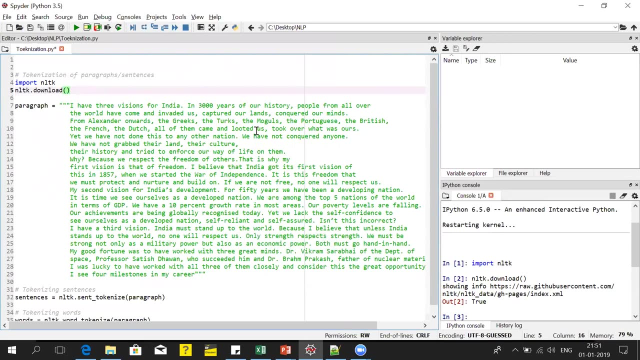 downloaded all, all, all the packages all together. okay, i'm just going to after that. what you do is that, after you download it, you don't have to download this library separately, so i can remove this. okay, once you download it, all the packages will get downloaded automatically. now, 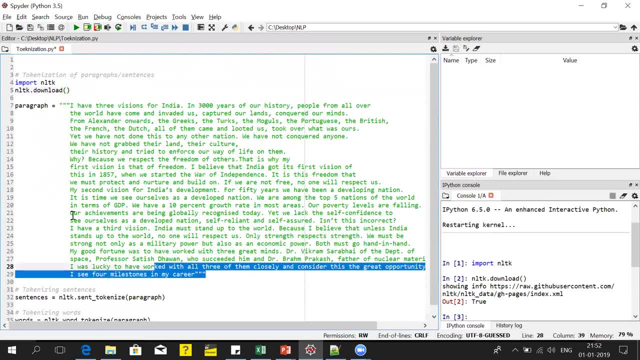 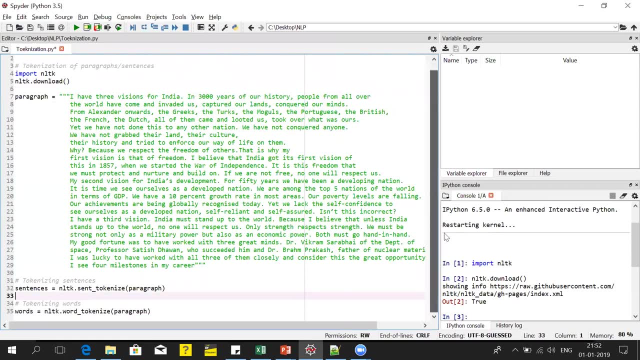 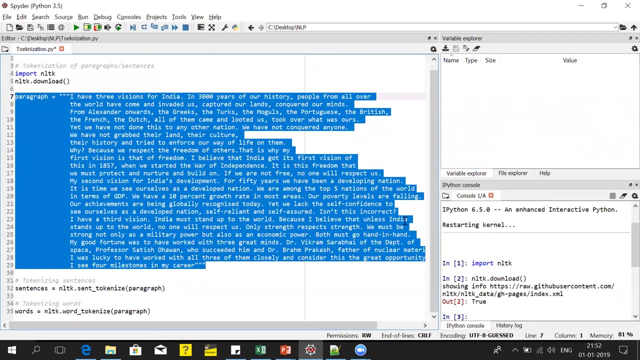 the first step of tokenization is that i will always be having a paragraph or a corpse. this is basically called as a corpse or a paragraph. then, once we take this paragraph, we have to convert this paragraph into sentences. in order to convert the paragraph into sentences, i will be. 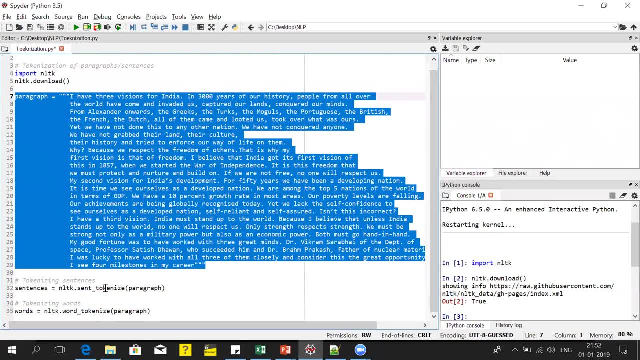 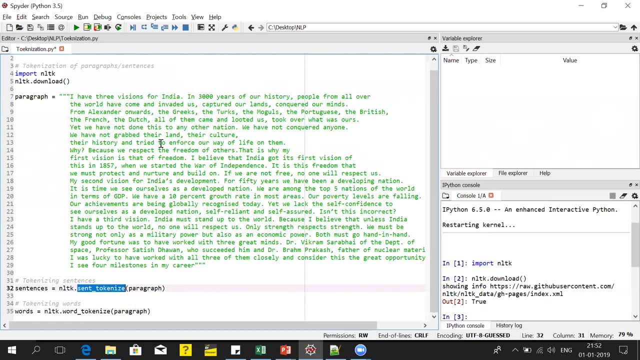 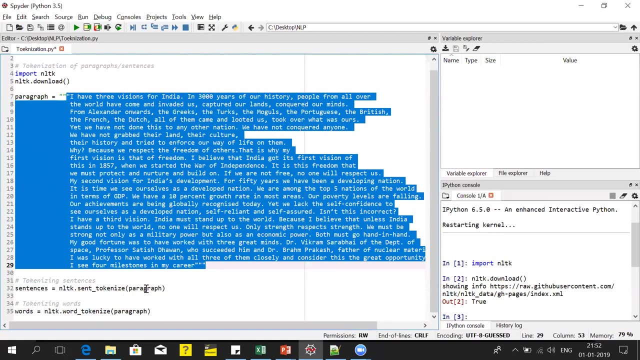 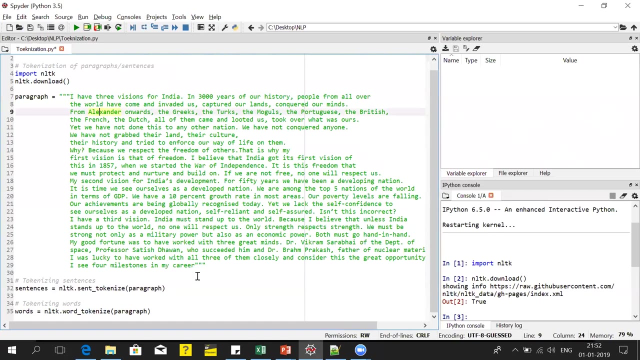 using an inbuilt function which is called as nltksent. underscore, tokenize, sent. and tokenize is a function inside nltk which takes the course, that is the paragraph, and it applies a lot of regular expression in below inside this function. this regular expression will be responsible in converting the paragraph into different, different sentences. so let me just execute this particular 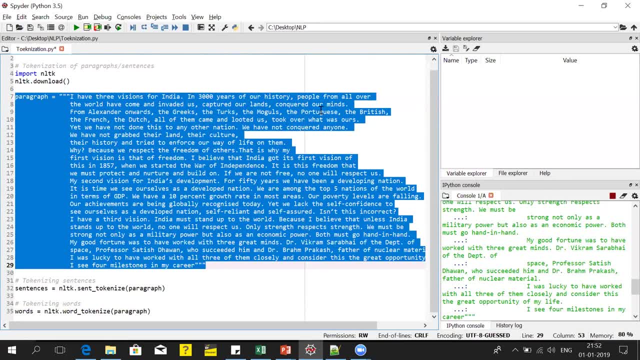 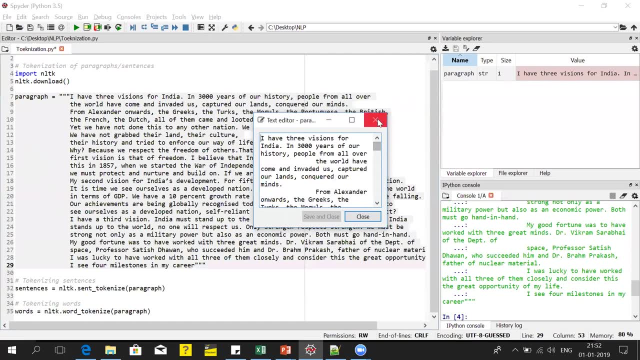 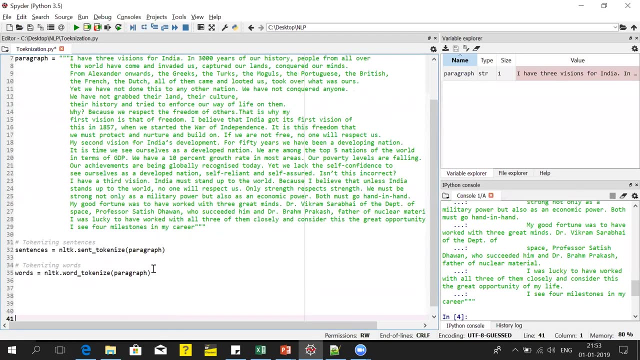 variable. that is my paragraph. once i execute it, you can see that the variable will be created with something called as paragraph, and this is my complete paragraph right now. the next step is that i will take up this paragraph. yeah, i'll take up this paragraph, and then i'll convert this into sentences by using the function that is present inside nltk. 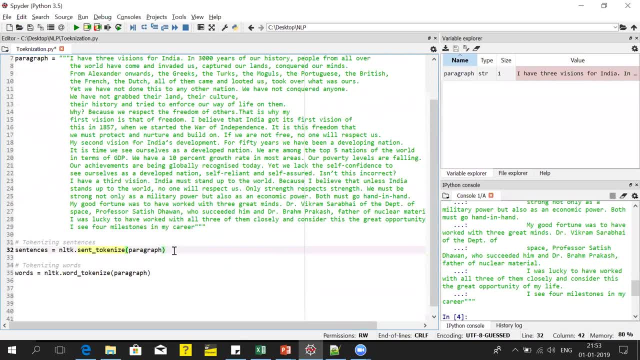 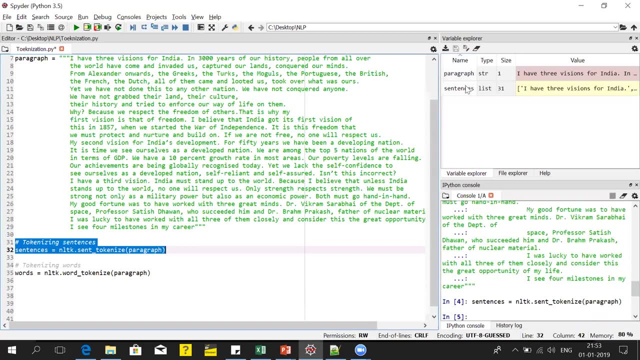 which is called as nltksent underscore tokenize. once i execute this, you will be seeing that all the paragraph, from all from this particular paragraph, the sentences will be taken and will be taken in the form of list. now, if i click on this particular sentences, you can see that. 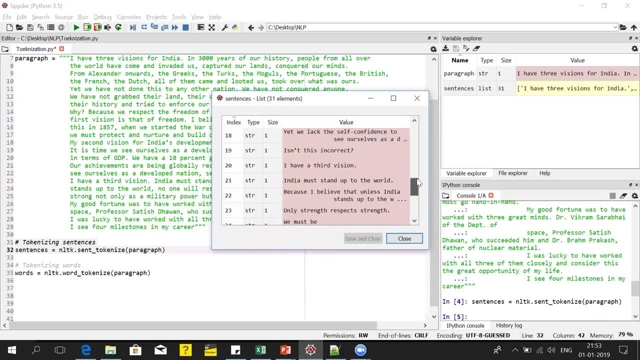 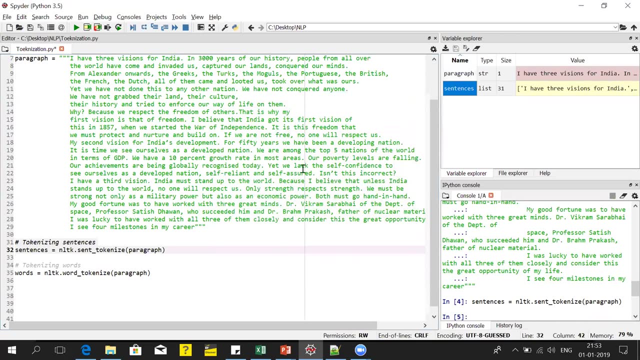 they are unique: 31 different lists, okay, so basically you can say that there are 31 sentences in this particular paragraph. now, after taking the sentences right, usually the text pre-processing usually happens on each and every word of this particular paragraph or this particular words or this particular sentences. right after we convert this into sentences, we will be converting. 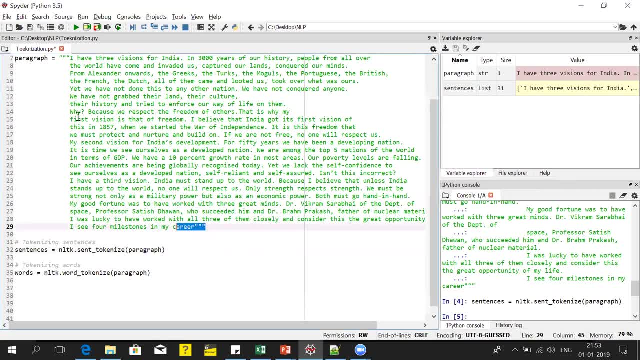 the sentences into words to find out how many total number of words are present in this particular paragraph. so for that i have a different function which is called as word underscore- tokenize. so word underscore, tokenize responsibility is basically taking all this, all this paragraph, okay, and this paragraph can be converted to word by word by using this word underscore, tokenize. 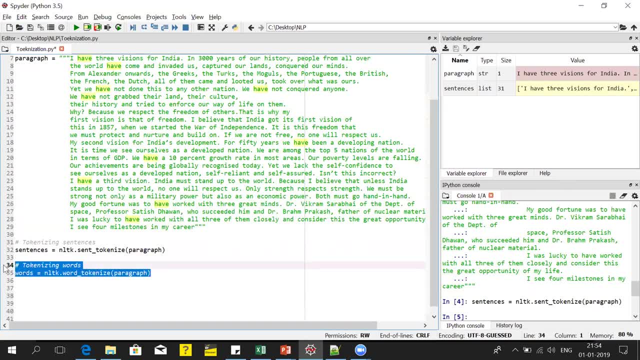 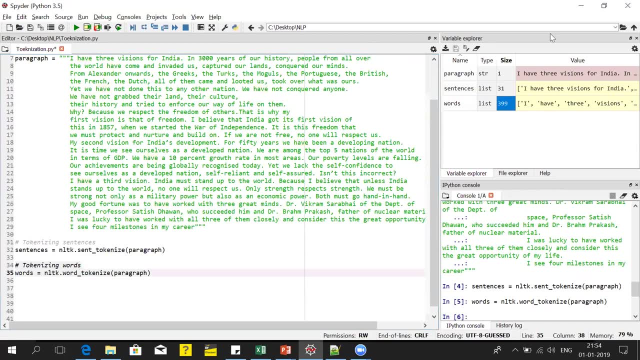 okay. so once i execute this, you can see that all i'll be having all the number of words that i have in this particular paragraph. so i have around 399 words. okay, 399 total words in this particular paragraph. then this will be in the form of list. now you can.